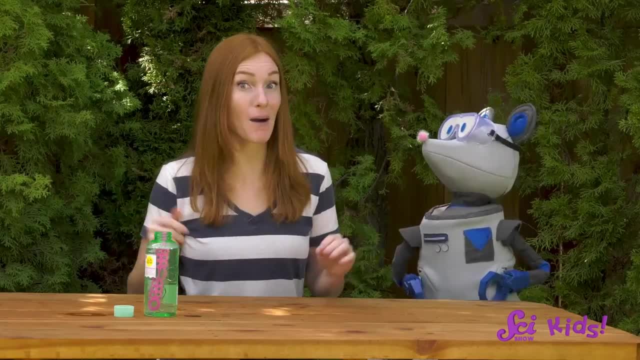 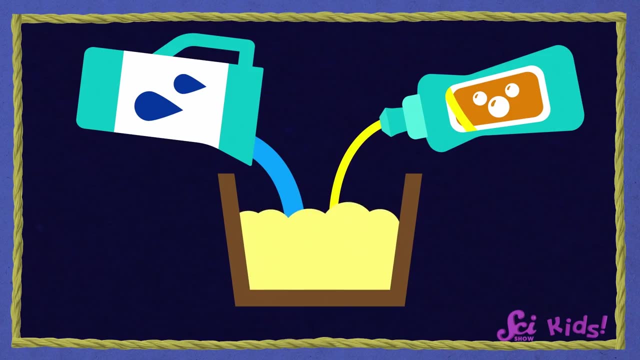 float around in the air, at least until the bubbles pop. Oh good question Squeaks. Why do bubbles pop? Well, water is really sneaky. As soon as you put it in a bubble, it tries to escape. And when the 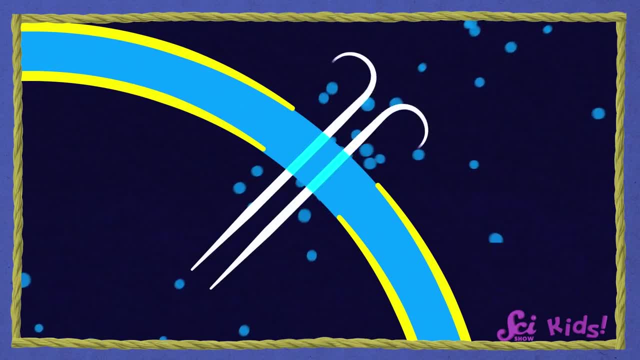 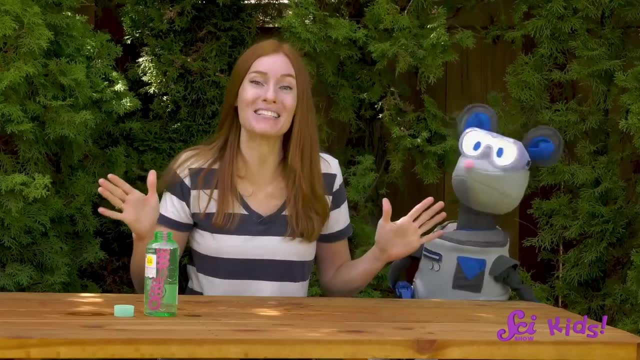 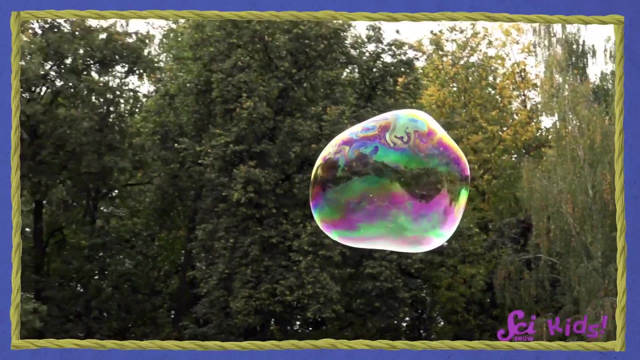 water gets away, the air trapped inside the bubble can follow it and escape too. And then what do you think happens? Yes, The rest of the bubble falls apart and it goes. pop The soap holds the water inside as long as it can, but eventually every bubble bursts. 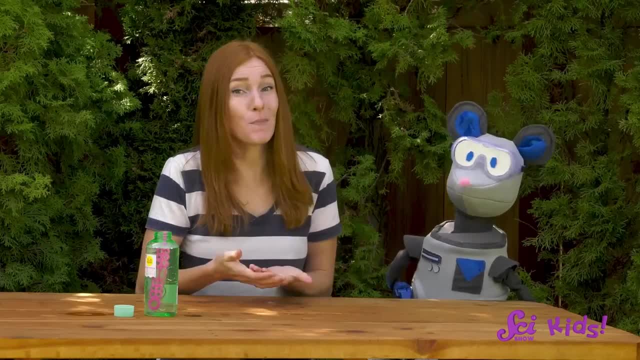 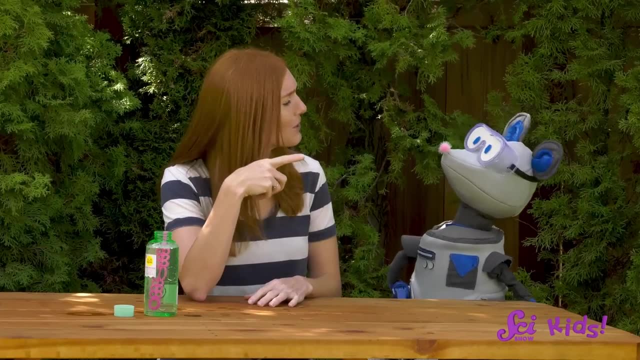 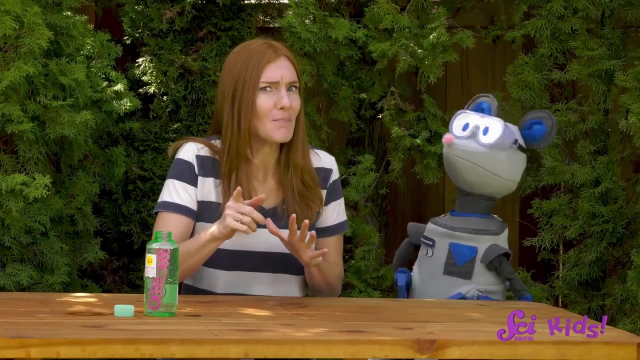 Oh, I know It is true, Soap bubbles do pop pretty quickly. An unpoppable bubble would be pretty fun. I wonder how we could make one. I know Let's try an experiment. I think if we make the soap thicker, maybe that will help to keep our bubbles around longer. There are lots of thick bubble soap recipes that we can make here at home. What do you think Squeaks? Should we try one out? We'll need four tablespoons of water and one tablespoon of dish soap, just like our first bubble solution. 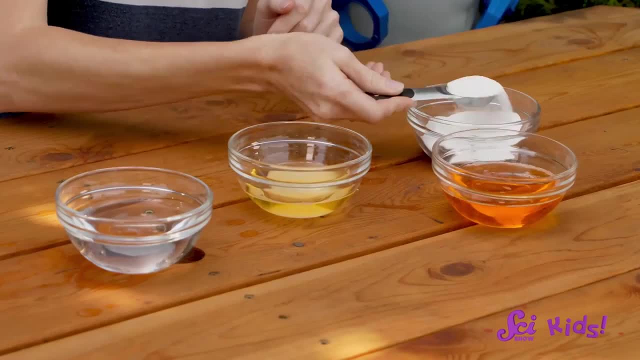 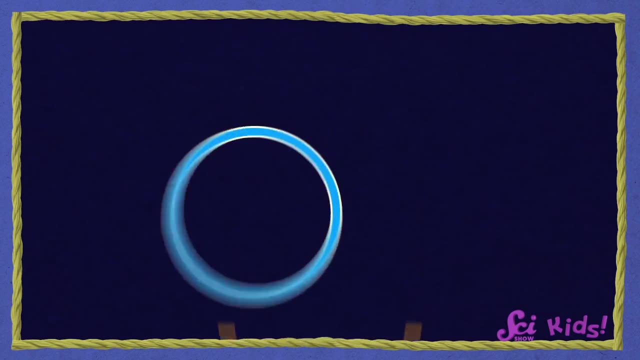 Now we'll add our special ingredient: two tablespoons of sugar. Oh, good question. The sugar should help the bubble. It's going to help make the soap layers of our bubble really thick. I'll stir until I can't see the sugar anymore. 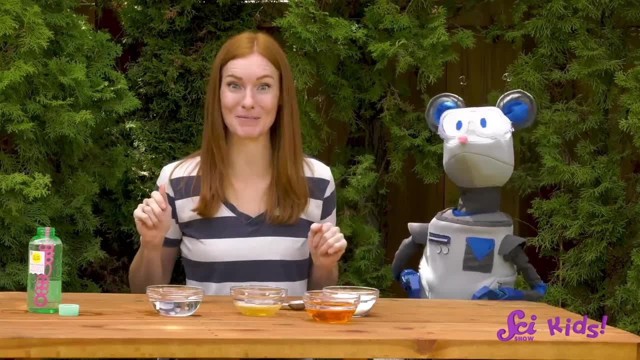 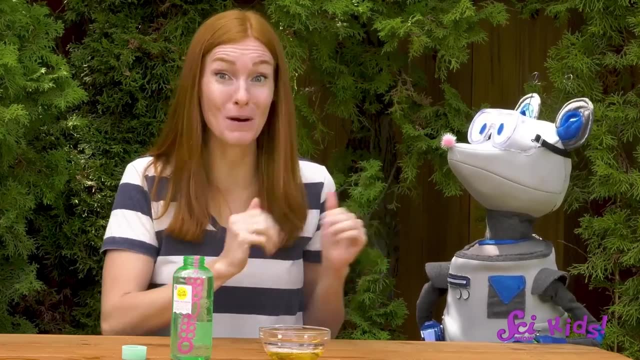 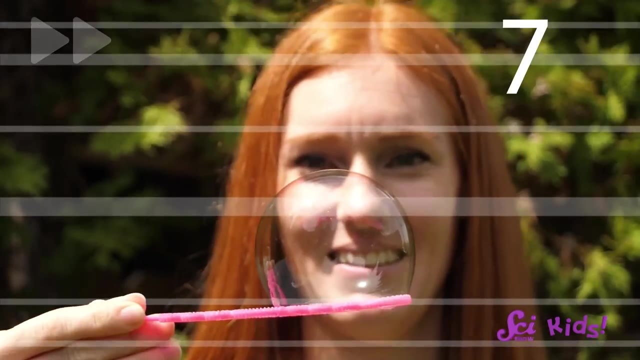 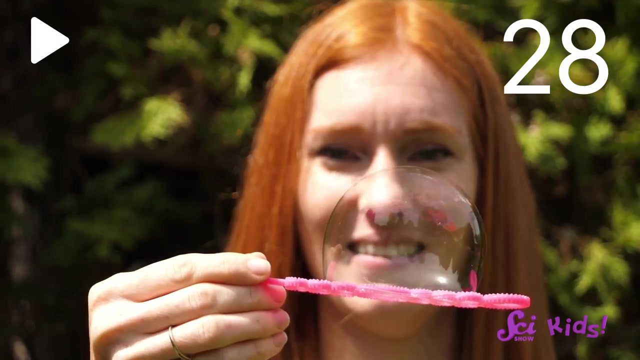 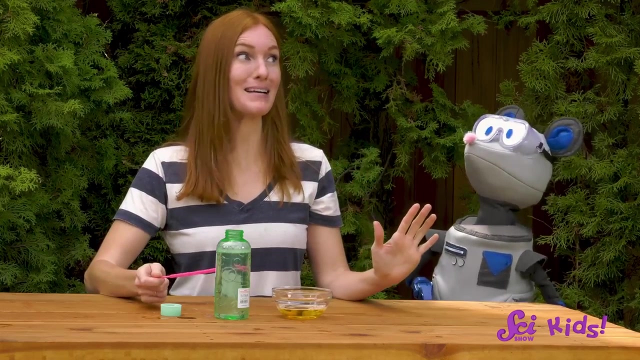 All right, It's time to compare our bubbles. We'll count how many seconds it takes one of our old bubbles to pop and then see how many seconds it takes one of our new bubbles to pop. First our old bubble. Wow, Not bad, That bubble lasted 30 seconds. 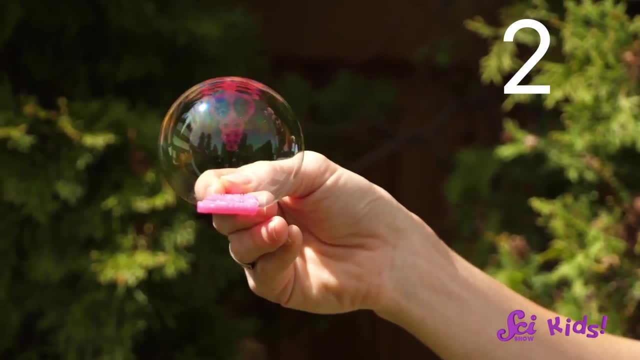 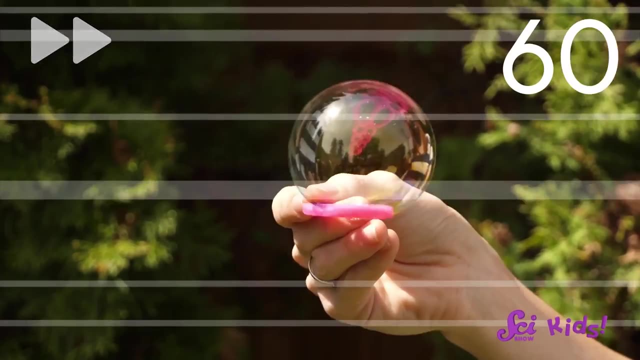 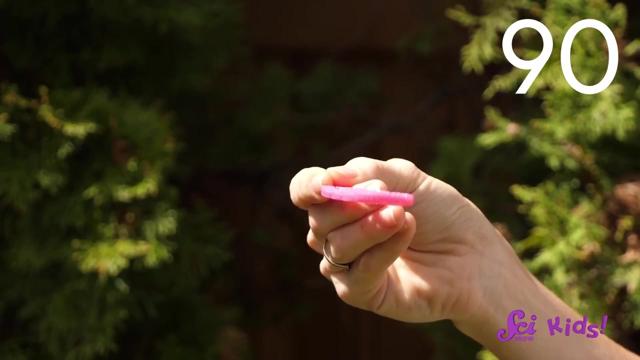 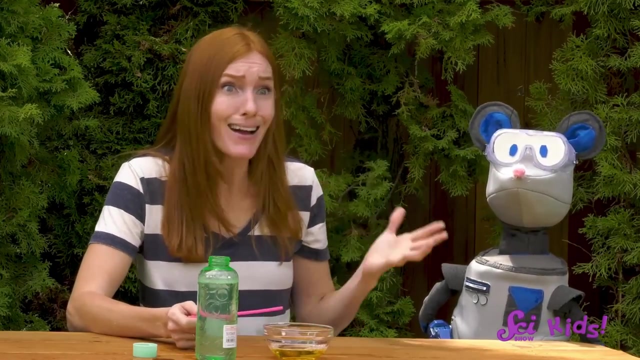 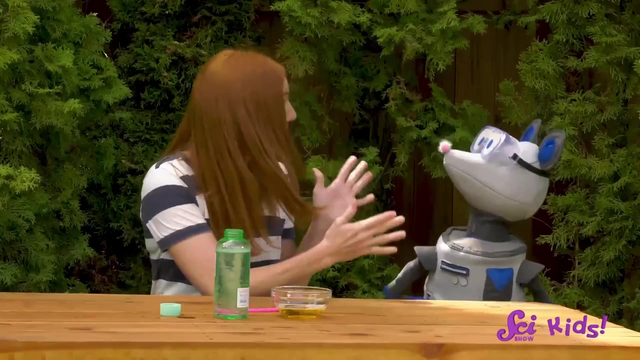 Now let's see how the thicker bubbles do. Wow, That bubble lasted way longer. The thicker bubble lasted 90 seconds. That's 60 seconds longer than the bubble without any sugar. Ooh, I would love to do more bubble experiments. 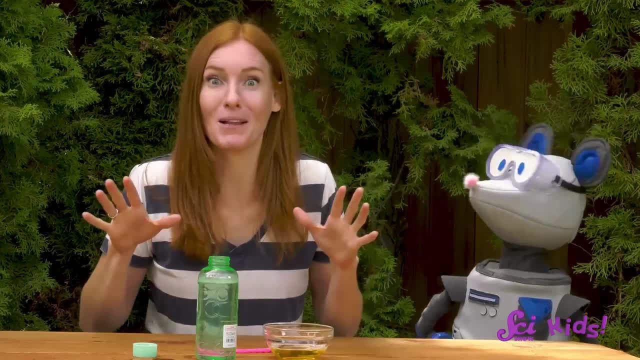 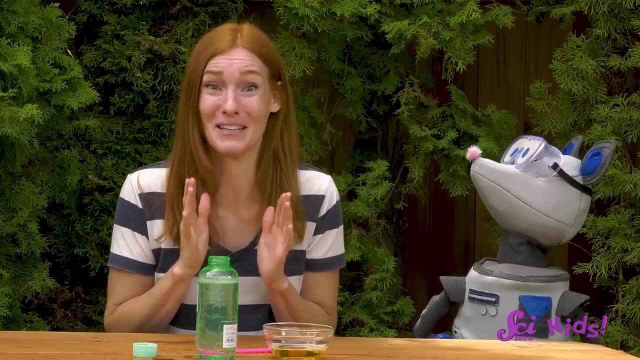 There are lots of bubble recipes we could try. We could replace the sugar with something like corn syrup or glycerin And, if we get our hands wet, we could even try holding the bubbles. How long do you think you could make a bubble last?